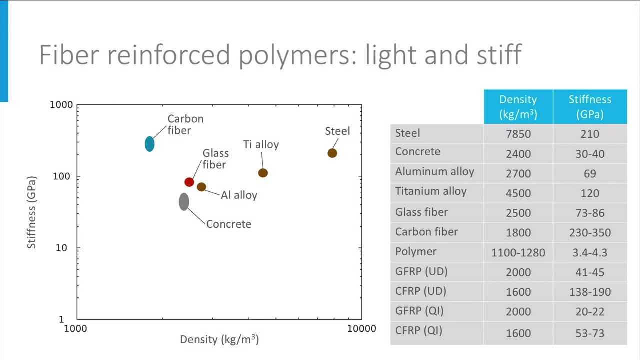 are for the stiffness in axial direction. Carbon fibers have different stiffness in different directions. The axial direction is the stiff direction, but also the most relevant one. Carbon is close to our ideal material, stiffer than steel, lighter than aluminum. The properties of glass are also good. 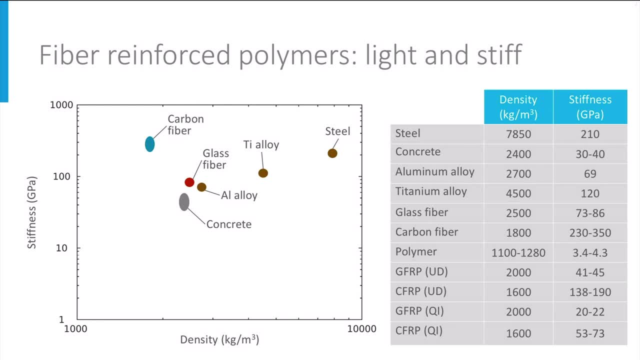 However, these values are for the fibers only. Fibers have to be combined with a matrix material to form a material that can be used for structural applications. In FRPs, the fibers are combined with a polymer matrix. The polymers that are used: epoxy, polyester, maybe a thermoplastic like PEEK. 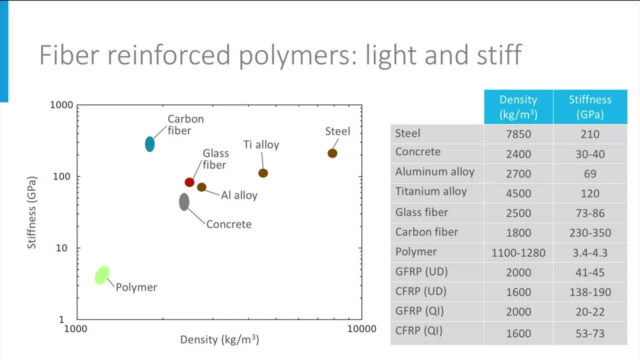 are all very light, with the densest density of the material. They have a density between 1100 and 1280 kg per cubic meter. but their stiffness is also much lower than any of the other materials in our chart. So for FRPs to have a good stiffness we must have a high fiber content. 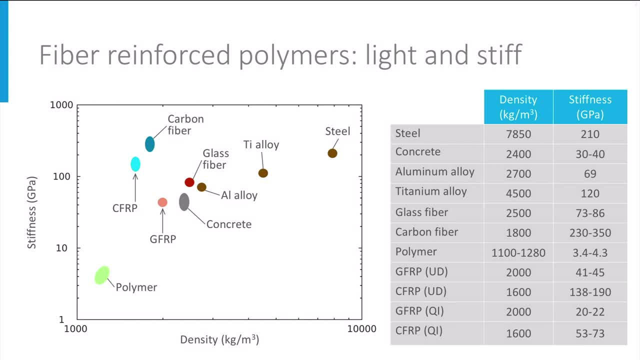 The composite stiffness is obviously going to be lower than the stiffness of the fibers. The good news is that the weight will also be lower, especially for GFRP. The FFRP is the same as the FFRP with the heavier glass fibers. 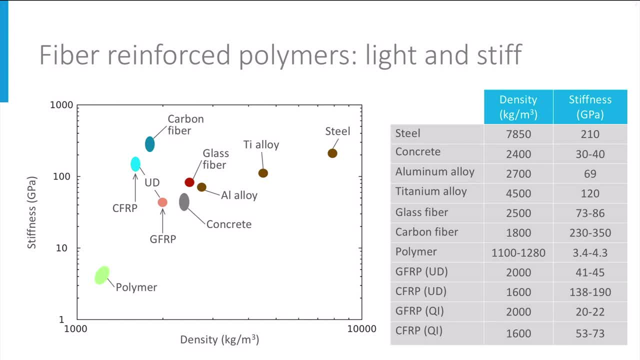 This is not the end of the story. These properties are for unidirectional FRP composites that have low stiffness and strength in a direction perpendicular to the fibers. To mitigate this weakness, laminates are made layered structures with different fiber direction in the different layers. 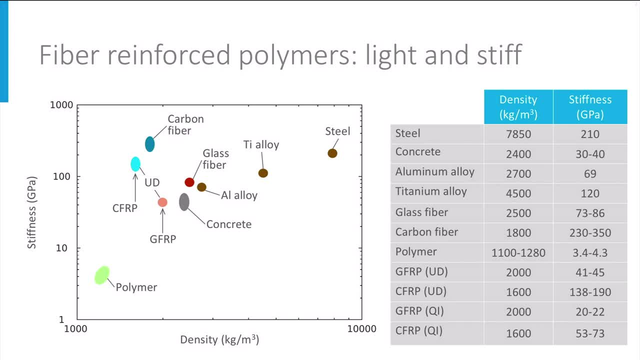 Depending on the application, the fiber distribution can be UD dominated or it can be such that the laminate has equal properties in all directions. This last extreme is obtained with a quasi-isotropic layup. If we also include the quasi-isotropic layup in the chart, 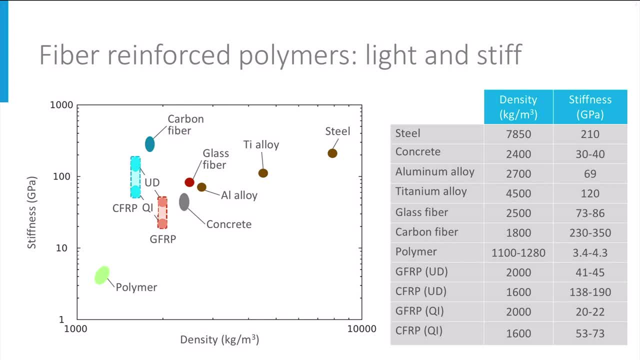 we see that the performance is less impressive. For a real FRP design. the stiffness in primary load carrying direction can be in between the UD and the quasi-isotropic values. A stiffness in one direction that is higher than the quasi-isotropic one. 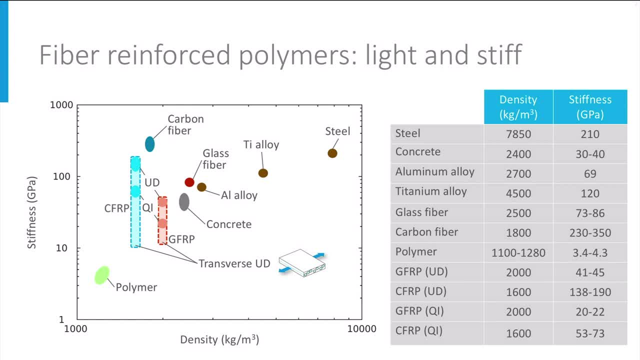 is going to have negative consequences for the stiffness in other directions, which will be even lower than the quasi-isotropic value. One more point of attention is that the out-of-plane shear stiffness of laminates remains low, irrespective of the fiber orientation in the layers. 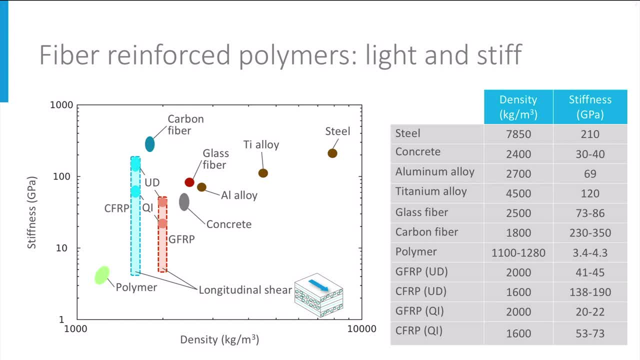 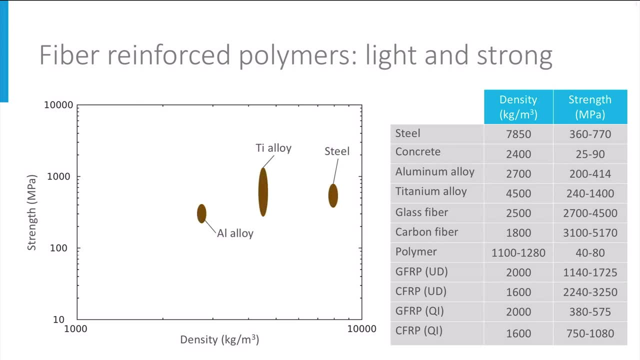 In any case, there are no fibers in the direction of this shear stress. If we remake this chart for strength, the relative location of the metals is similar, with a strength of 370 to 770 MPa for steel and 200 to 414 for aluminum. 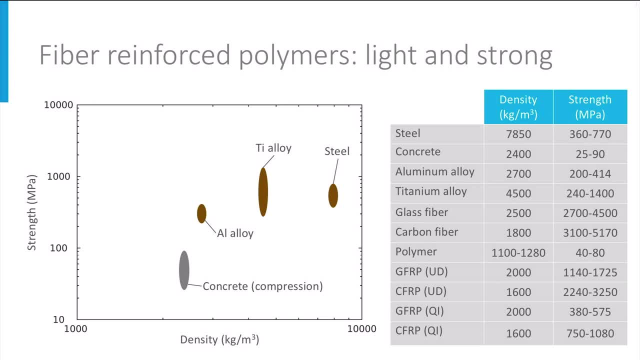 The strength of concrete, even the compressive strength, which may go up to 90 MPa, is significantly lower than that of the metals. The polymer matrices that we use have a strength in the range of 40 to 80 MPa. 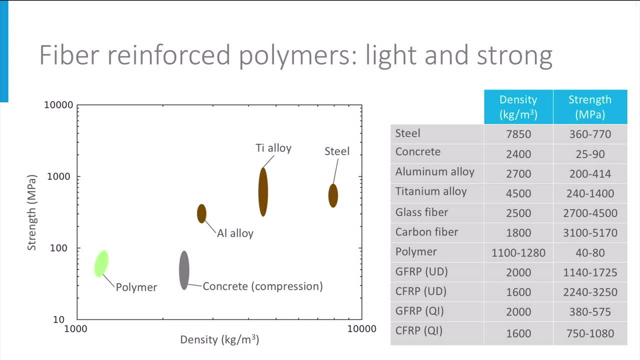 accounting for the low weight. that is already good. The fibers are performing really well when it comes to strength. Both glass and carbon have a much higher strength than the classical engineering materials, at 2700 to 5000 MPa When combining fibers and polymer, the strength that can be reached in UD FRP. 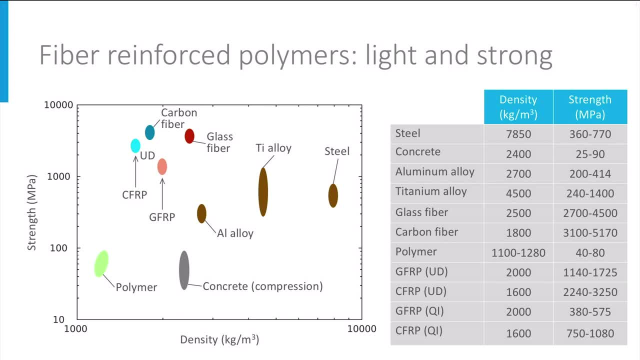 is still higher than that of steel at 1000 to 3000 MPa. So for strength, the comparison between FRP composites and traditional materials is more favorable than for stiffness. However, here too the material behavior is directional. The UD material is weak in transverse direction. 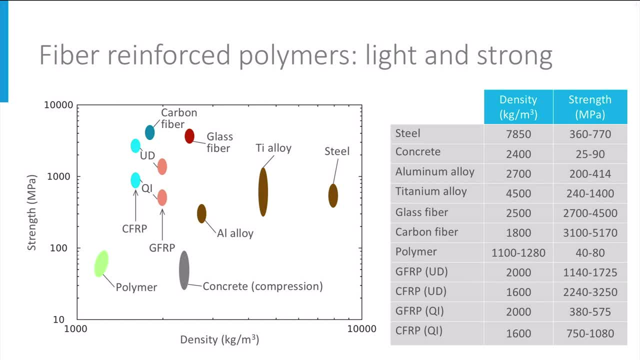 In multi-directional laminates, the strength is lower than in the UD material. In all cases, the interlaminar strength remains high, hence low. Moreover, we have been looking at tensile strength. The compressive strength of FRPs is typically lower than this tensile strength.